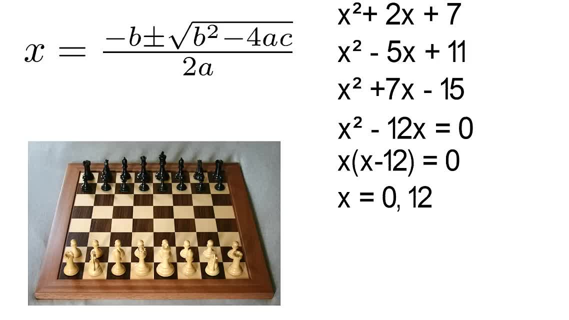 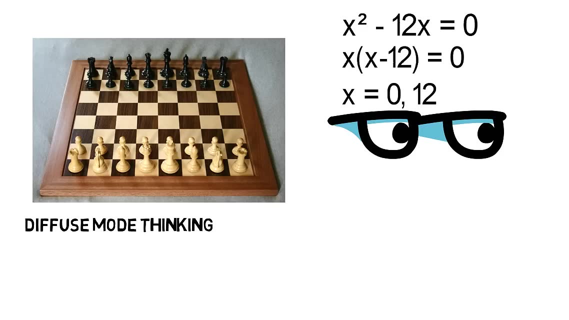 of what move they should do. They try to continue to scan the board for better moves. however, through studies of their eyes, they've shown that their focus stays on the original move they thought of. And this is where diffuse mode thinking comes in. It allows your brain to relax and the 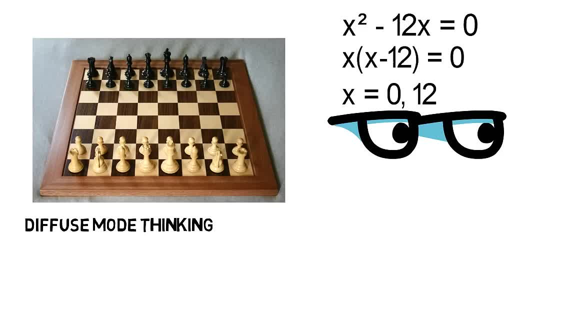 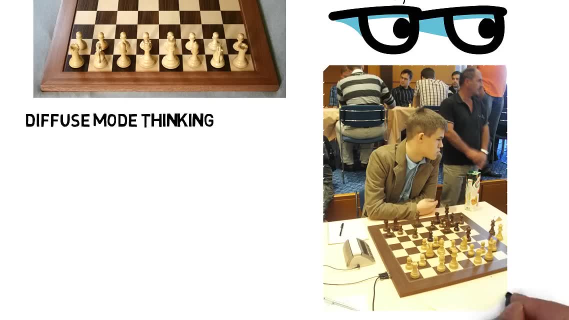 neurons to connect and kind of work in the background which allows you to see more of the big picture. In the book the author shows a picture of a chess grand master during a game, who gets up from his seat and looks away from his game. He takes a short amount of time to distract. 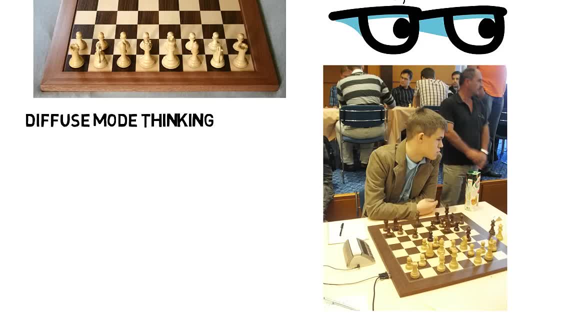 himself and let his mind wander, so he doesn't become stuck in a narrow way of thinking- And this is what diffuse mode thinking really does. You just take a break from that and get back into focus. Then when you come back to the problem you'll have a fresh mindset and often the solution. 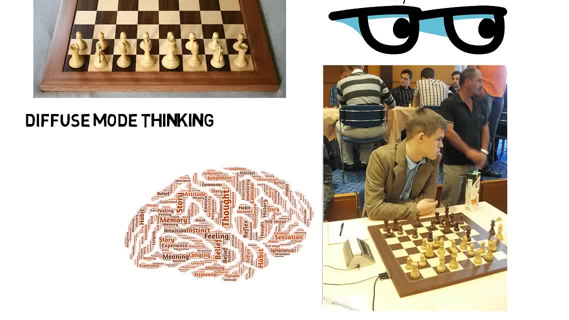 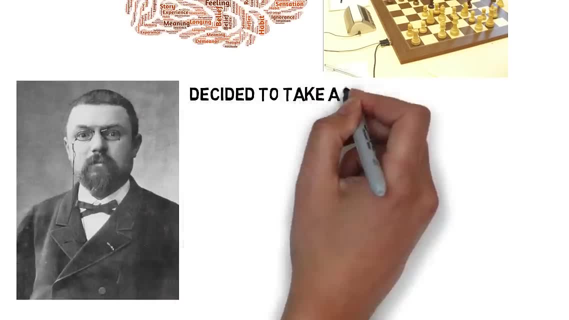 or a better solution comes to you much faster. A very famous French mathematician, Henri Poincaré, struggled to crack a difficult problem, so he decided to take a vacation, And when he was getting on a bus the answers suddenly came to him from a part of his brain that continued to work on the problem in the 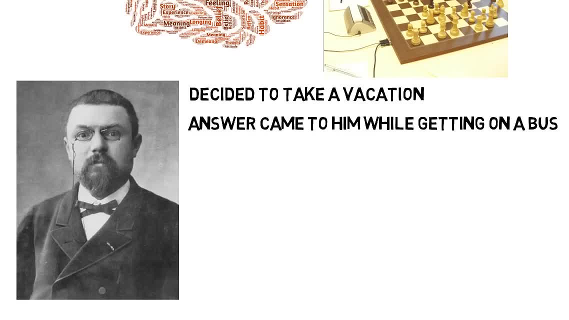 background And you'll hear of many stories where this kind of thing happens. So this is the foundation for improving your skills: You need to have an understanding of where you're going and how you're going to go. You need to have an understanding of. 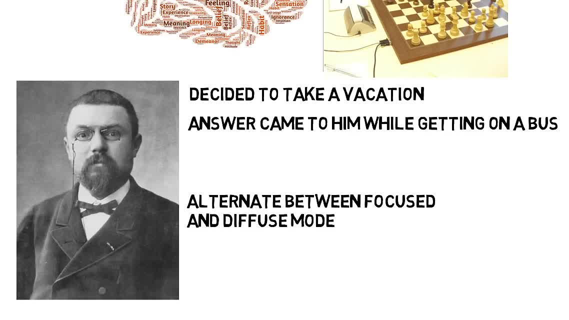 to alternate between focus mode, learning and diffuse mode. No, you cannot just let your mind wander and wait for the answers to come. You need to focus intensely on a problem. then, when you are stuck, take a break for maybe two minutes, maybe an hour, and then. 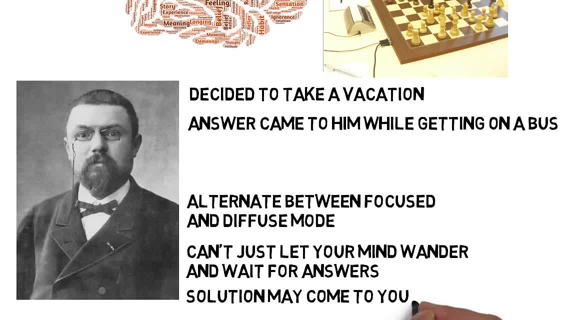 come back and focus again and the solution may come to you much quicker, as you have a fresh look at the problem. It may not just happen like it did for this mathematician, but resume the problem and it may surface faster than you think. Ways to get into diffuse. 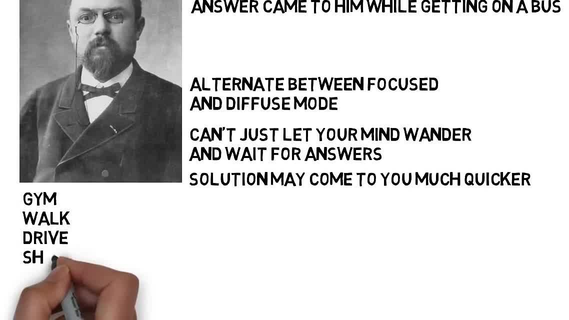 mode include going to the gym, going for a walk, going for a drive, taking a shower, sleeping and much more. And remember you can't just look at a problem you have no clue what to do on and then take a break and think you'll get to the solution. You have to be. 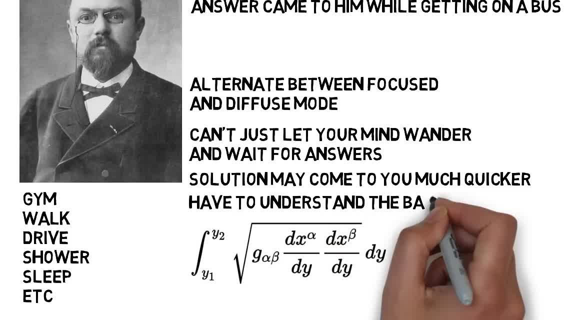 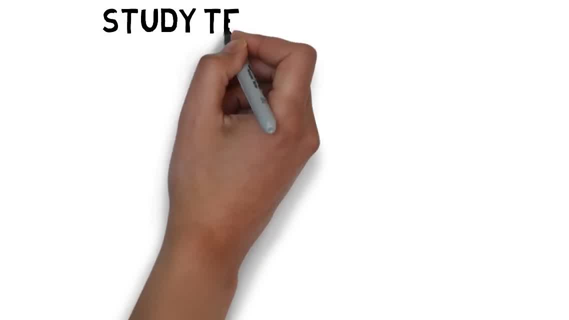 logical. You need to actually understand the basics, then focus on the problem and then alternate between that focus and diffuse mode thinking. Now let's get into some more specific study techniques and tips When it comes to learning math and science. learning fast is. 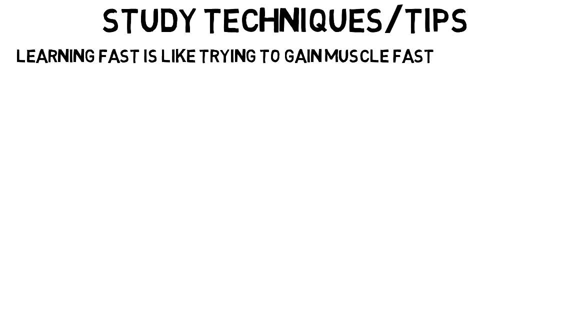 like trying to get the answer to a question. When it comes to learning math and science. learning fast is like trying to get the answer to a question. When it comes to learning math and science, learning fast is like trying to get the answer to a question. When it comes to learning math and science. 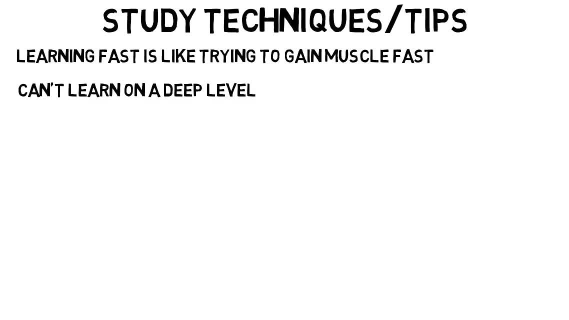 you can't learn on a deep level in one or two nights. You start over. so you have to understand the Ter] rule and if you're able to memorize it going forward, then you actually learn a little earlier. So those are some tips to keep you visual on your own. 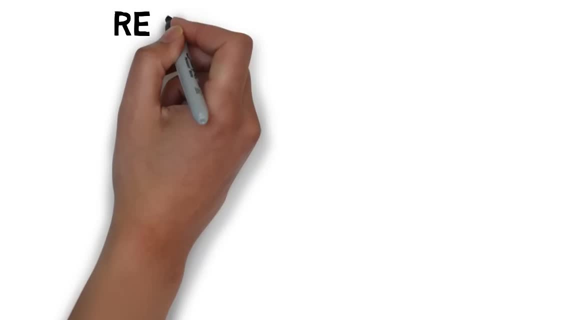 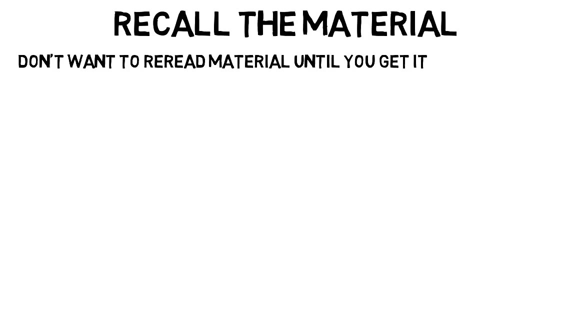 subject matter supplies and ways to use your brain. It's best to learn a little everyday to make sure learning is anybody's Younger and effective for recuperative learning. There are even exercises into health and wellness that help with your ability to pick up knowledge on theah stuff. 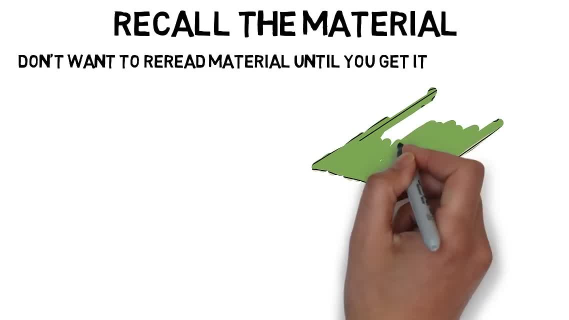 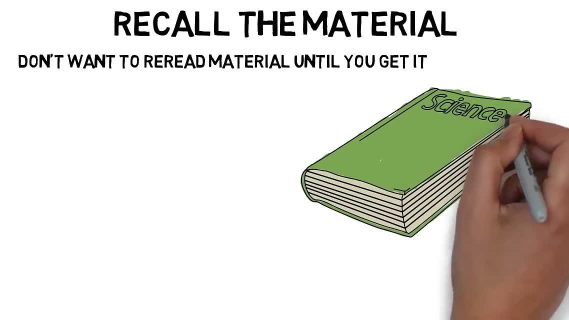 But what you DO want to do is read something new and turn away or close the book before and try to recall what you just read as much as possible. Then read it over again and repeat that one more time. They found just with two repetitions. 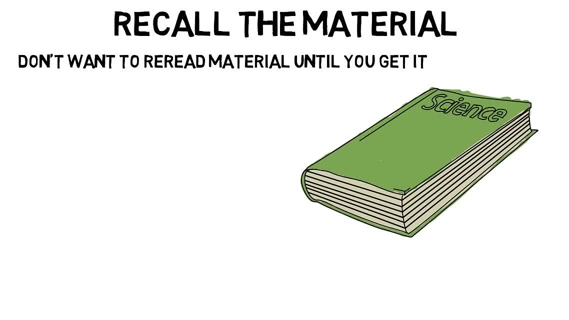 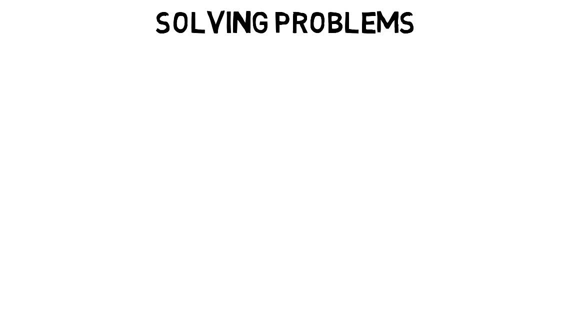 this worked better than nearly any other method done in the same amount of time. But okay, what about when it comes to doing problems like in math, physics, engineering etc. which aren't just memorizing things? Again, here's what you don't want to do. 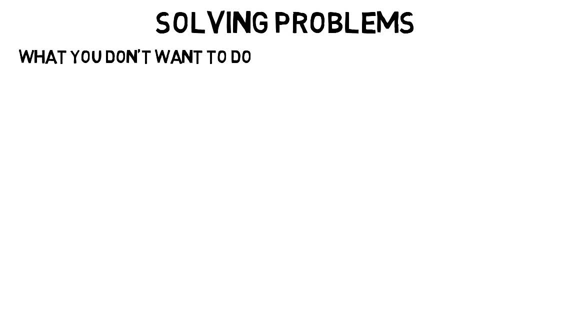 and this I thought was very insightful because I know it will apply to a lot of people watching. What you don't want to do is attempt a problem. then when you don't understand it, you look at the solution and say, oh, I see how they got that, and then move on. 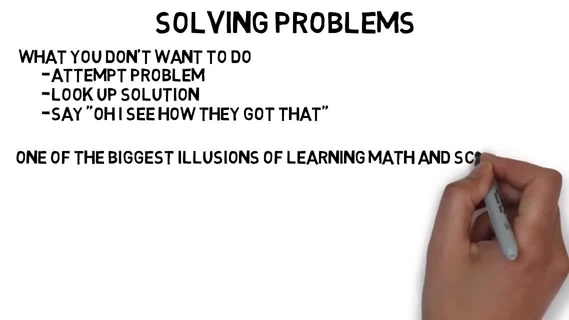 This is one of the biggest illusions of learning math and science out there, so you should not fall for it. You haven't learned the concept, even though you think you may have. If you need to look at the solution, that's no problem. 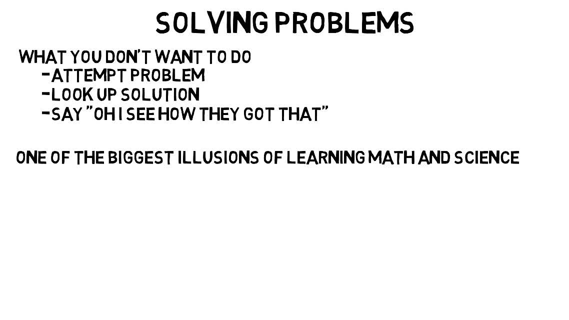 but then you need to do a totally different problem on that topic and solve it completely on your own. So if you are struggling to learn a new concept, what you want to do is first read about the topic and make sure you understand the fundamentals. 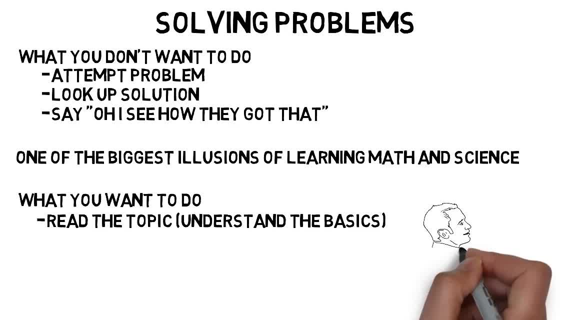 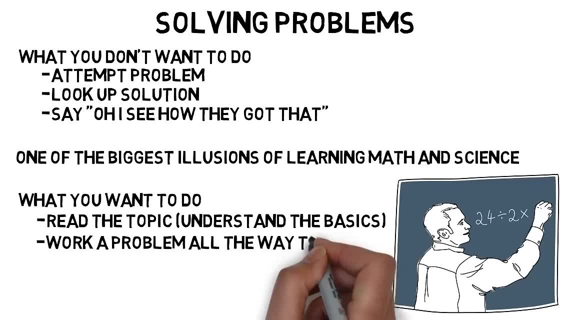 Ask your professor, your friends or whatever it takes, so you can just get the basics. You don't just want to dive into problems without learning the fundamentals. Then what you want to do is work a problem all the way through, Try to have the solution available, but don't look at it unless you really need to. 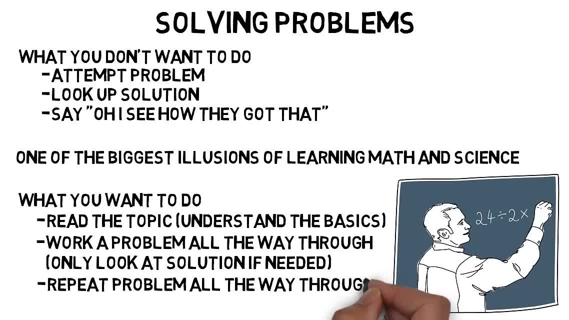 Then if you didn't fully understand the problem, you need to repeat it all on your own And make sure, as you're going through each step, you understand why it's being done, not just how it's done. This allows your brain to make connections. 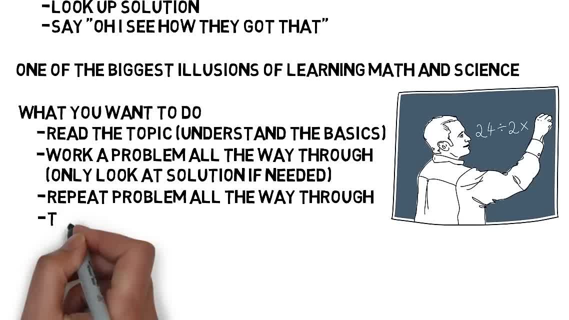 rather than just reading the solution and thinking you have it. Then you want to take a small break after a few problems, Go into that diffuse mode thinking so you can come back with a fresh mind. And if you don't get something, you need to practice it a lot. 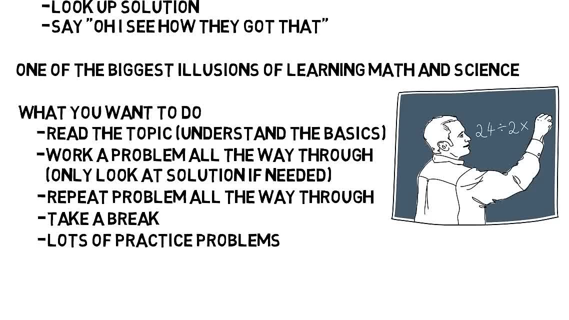 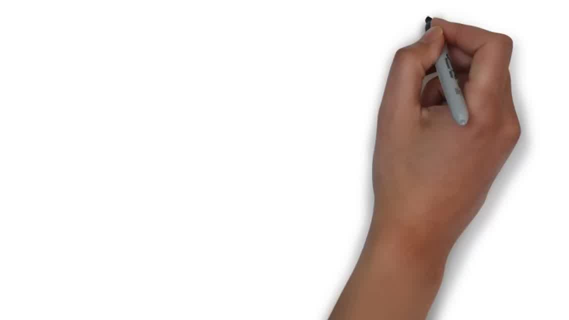 That's basically what this all comes down to. It will take time, but your brain is going to keep making connections, especially as you accomplish problems on your own. Now, many students, on the other hand, will do a certain math problem correctly, but then, right after that, they'll do more of those same problems. 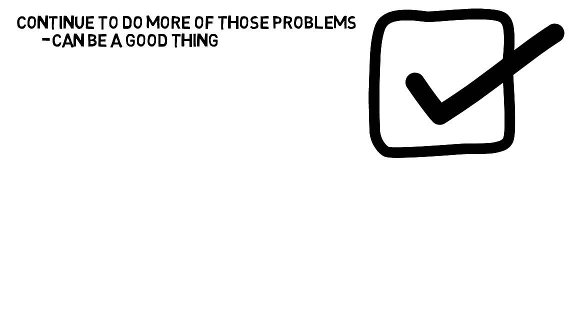 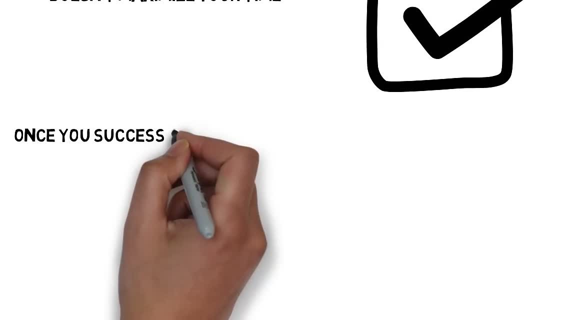 Now, this can be a good thing- and improve test scores for sure- but this doesn't maximize your time in the most efficient way. If you want to learn the most in the shortest amount of time, then once you successfully learn a concept and do maybe a couple problems correctly, move on. 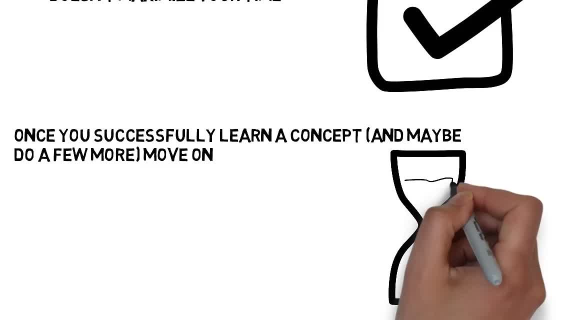 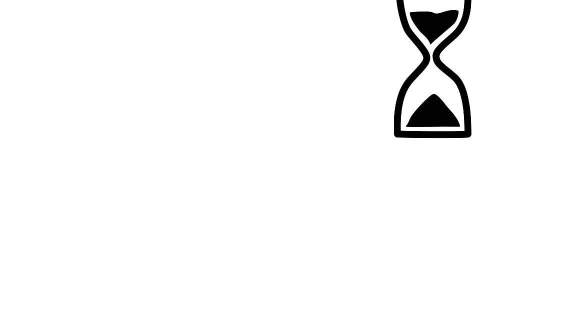 If you had all the time in the world, then of course, practice as much as you can, But often that's not the case. so this is something to keep in mind. And another tip which I really thought was interesting was to mix up the sections of the book you're doing problems in. 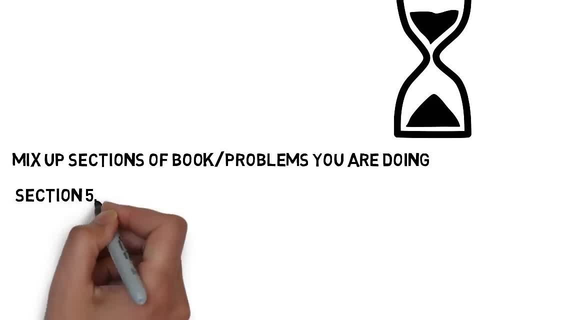 Like, let's say, your homework is in section 5.4 of the book. We'll do some of those problems, then do some from 5.3, then go back to 5.4, then maybe go back to 5.2.. 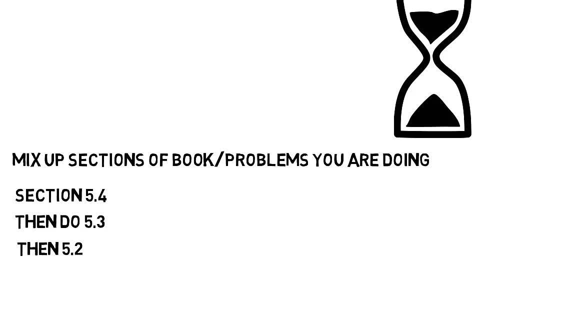 Especially if you're struggling. you'll need this practice Now. why do you do this? Because you want to make sure that you could do all these problems on a test if you didn't know what section things were on. If section 5.4 is all about synthetic division, 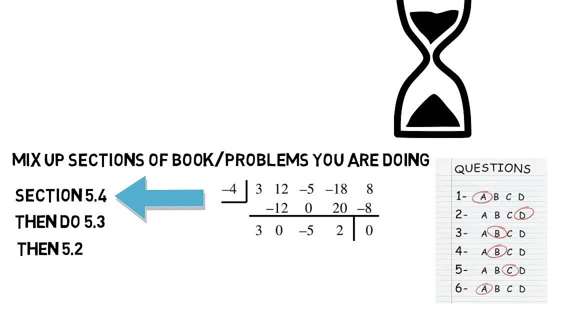 even if you get an abstract problem, you still can assume it requires synthetic division. But just given that problem randomly on a test, would you know to do that? This is something to ask yourself and a reason to kind of mix up the sections you work on. 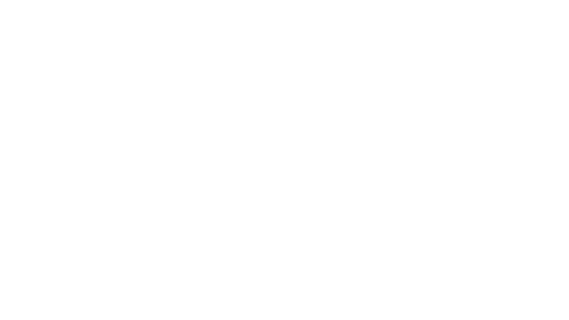 so that you can fit the pieces together Now. in another video I talked about procrastination, but this book had a few takes on it as well, and I wanted to offer some more advice for those who have issues with procrastination. One thing to try is the Pomodoro Technique, which there are many videos on. 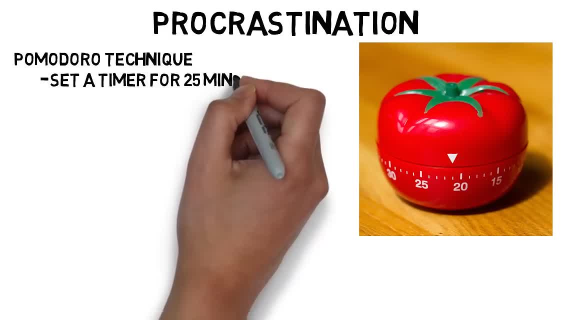 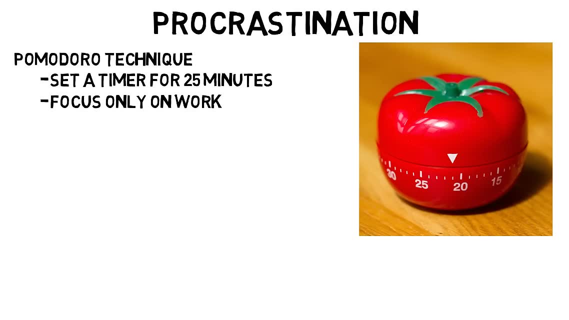 but essentially, to sum it up, set a timer for something like 25 minutes, maybe a little less or more, but then solely focus on work for that time. This is short enough where anyone can really focus for that long. Then afterwards reward yourself with some internet surfing or texting or whatever. 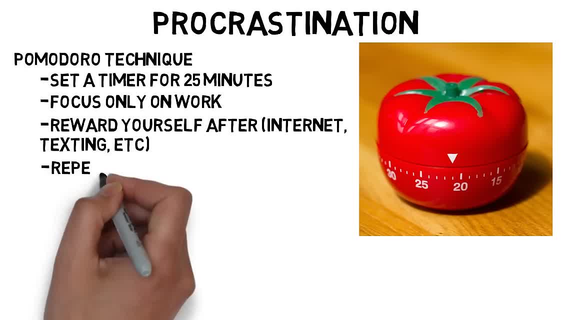 but not for too long. maybe just a few minutes and then repeat the process. Some people argue that they feel rushed with a timer in the background when doing something like math, But studies have shown that this actually helps because it will make you become accustomed to being on the clock. 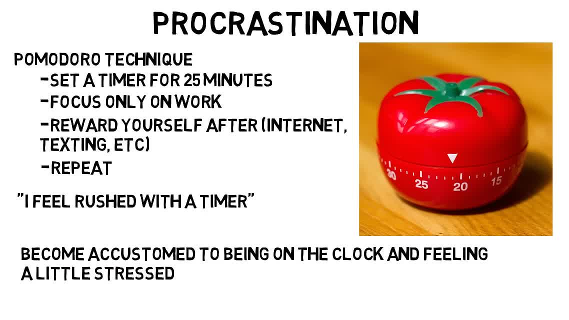 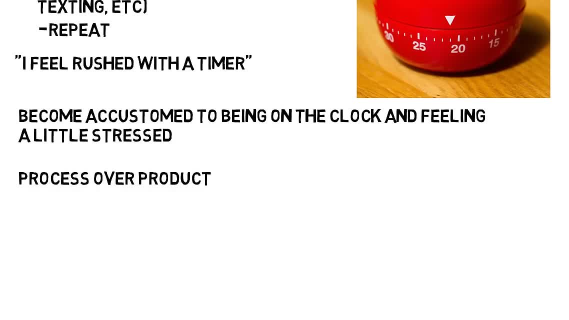 and feeling a little stressed, so that when you're taking a test and that stress occurs, you're able to perform better. Also, you want to make sure you focus on the process, not the product, As in, you should care more about the time you're putting in. 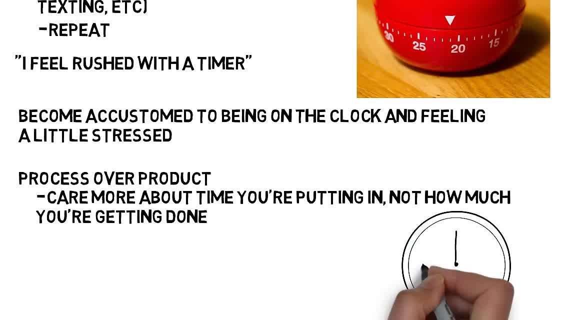 not how much you're getting done. It doesn't matter if it takes two or five hours to complete your homework, assuming you have the time. you really want to make sure you understand the material on a deeper level and learn how to apply it. 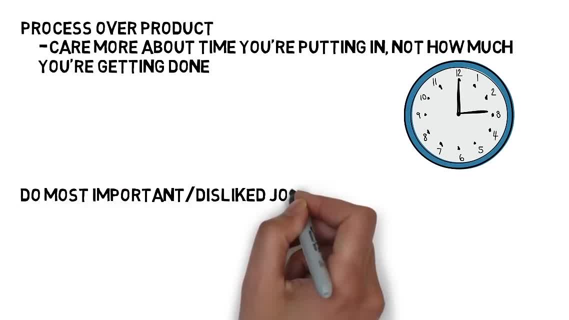 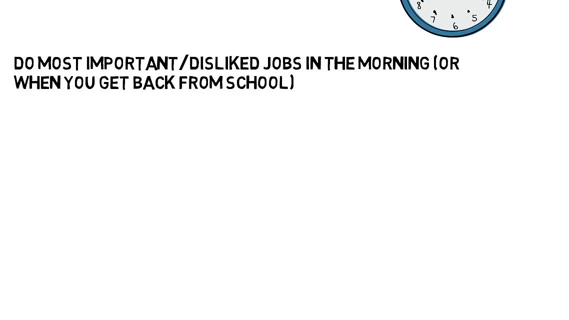 Another very effective tool is to do the most important and disliked jobs in the morning when you get up or maybe immediately when you get back from school. This then gives you that momentum to keep going. Another thing to try is mental contrasting, where you basically picture where you want to be compared to now. 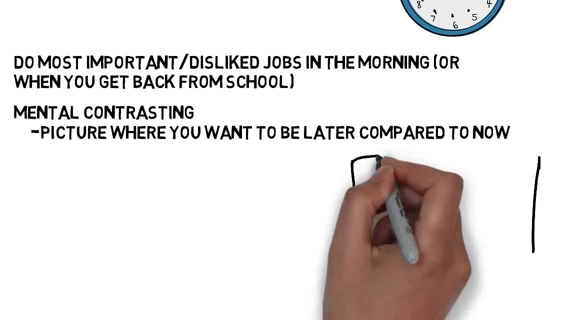 and why you are doing this. One student from the book was quoted saying that he put what his starting salary would most likely be on his wall and framed it to remind himself why he's doing all this work, and it helped him with procrastination- And I'm going to stop there with procrastination. 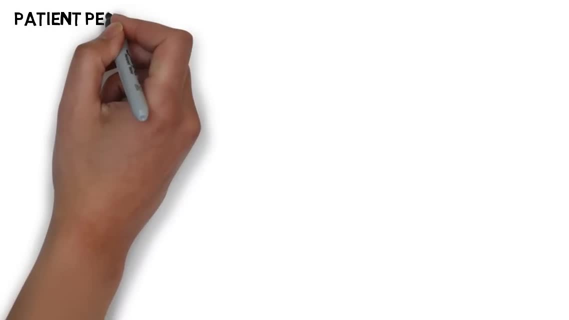 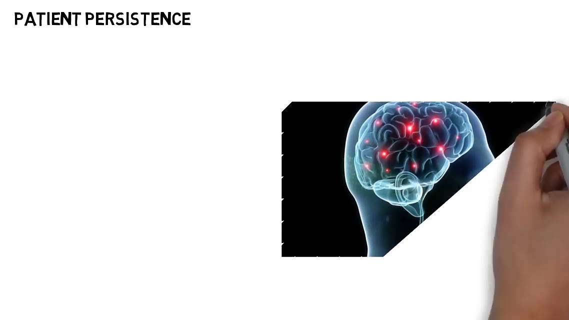 Now, when it comes to getting better at math or science, it basically all comes down to patient persistence. After so much time of doing all these techniques, it will reshape your brain and optimize the way you learn and solve problems. Persistence is often more important than intelligence. 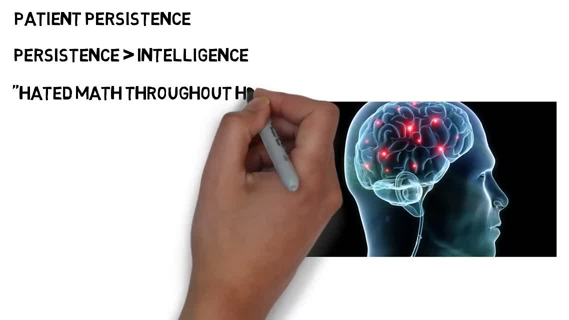 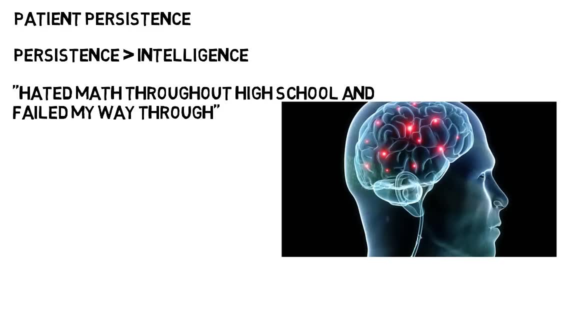 This author said that she absolutely hated math all throughout high school and failed her way through. She started studying just basic trigonometry when she was 26 years old, after being in the military, But she had a shift in her mindset and decided that she was going to get good at math.